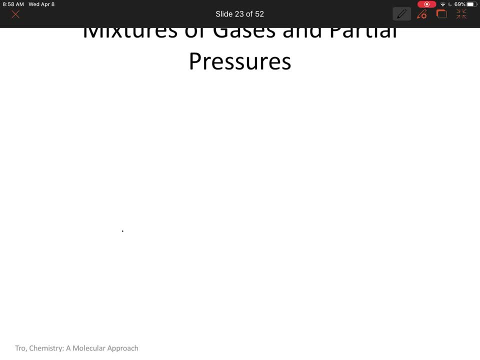 Mixtures of gases and partial pressures. So last little bit for talking about one more law and a few other equations about this chapter, for the simple gas laws and talking about gases, ideally until the second part of this chapter we talk about real gases and how the equations change a little bit. 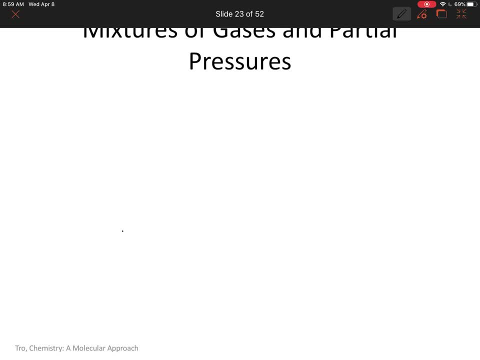 So basically, many gas samples are actually not pure. There are always little mixtures of other gas components that make that gas what it is: Molecules in an ideal gas. they don't come together and form something new, They don't interact. 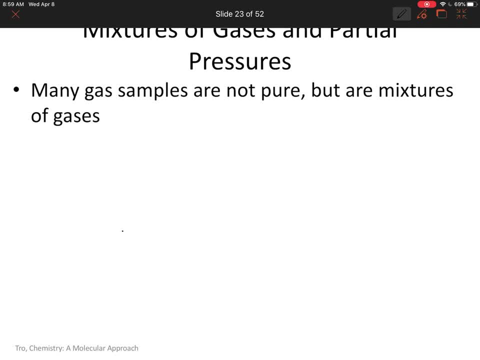 They are in the same container and constantly colliding with the surfaces of the container, but not colliding with each other to make something new. Thus each of the components in an ideal gas Make sure they act independently so they give off their own pressure to make this pressure of the gas overall. 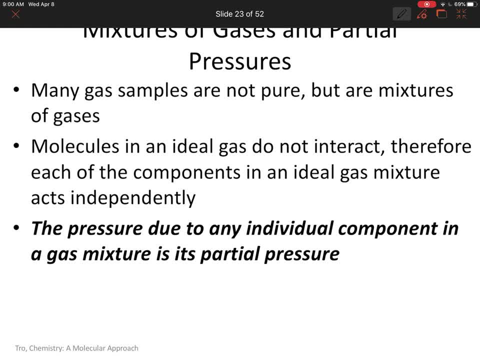 A great example of that would be air. so the air contains nitrogen molecules of around 78% of its pressure, and it's independent of the oxygen that's in air and the argon that's in air. The pressures that come from individual components in a gas mixtures are all called partial pressures. 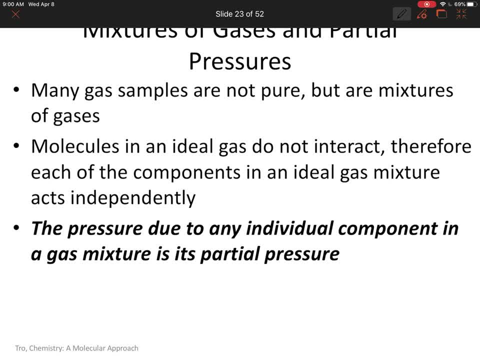 So, for example, air, the big pressure of air, the atmospheric pressure that we see, is composed of the partial pressure of nitrogen, oxygen and argon that it's made up of. That law is called the Dalton's Partial Pressure, and it's. the total pressure of a substance is equal to the partial pressure of however many components it has. 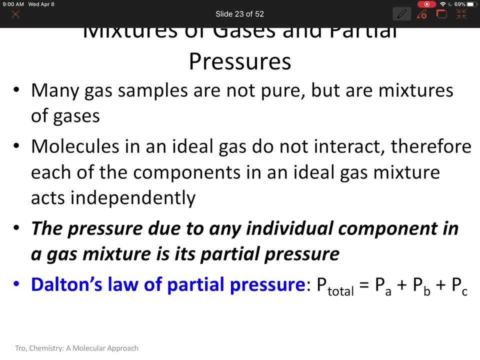 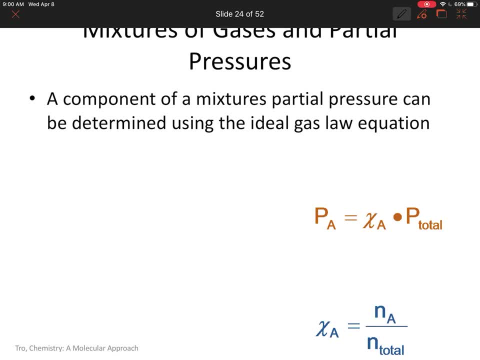 Here I have A, B and C. It could continue or it could be shorter than that. It just depends on how many components you actually have in the mixture. Here is my shotgun- motivation. So a component of a mixture's partial pressure can be determined using the ideal gas law equation. 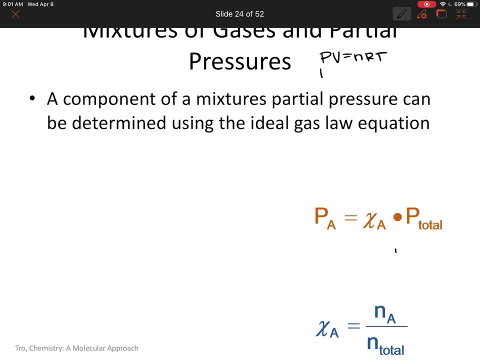 So you can. specifically, we know that the ideal gas law equation is equal to PV- NrT And I can say that this is my Pa And my moles of A that are contributing for me to get my partial pressure of just my substance a in the mixture. 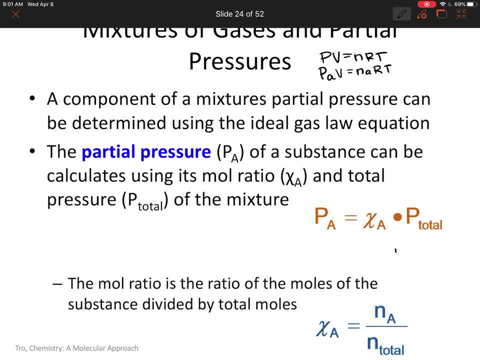 However, It can also be solved Another way, depending on the information you're given. The partial pressure P sub A, again P sub B, whatever mixture you're looking for of a substance- can be calculated using mole ratio and a total pressure of the mixture. 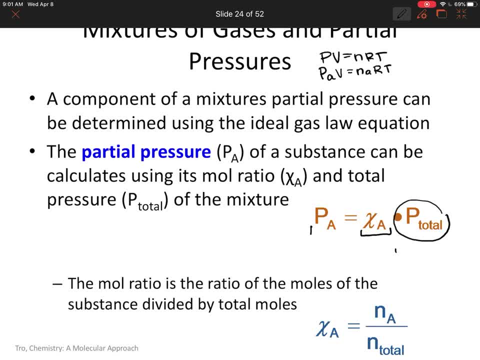 So, because we know that this is a ratio, if I multiply the ratio to the overall pressure of my solution, I can get how much that one substance contributed in pressure units. Well, how do I find mole ratio? Since it's a mole ratio, it will be the amount of moles. 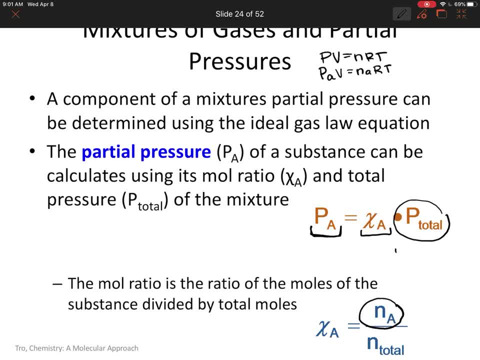 of that particular substance divided by the moles total. So you can apply these equations different ways depending on what you're looking for. If you are given all the information for a substance, that's total amount, you can find the pressure total using ideal gas law. and if you have the moles, 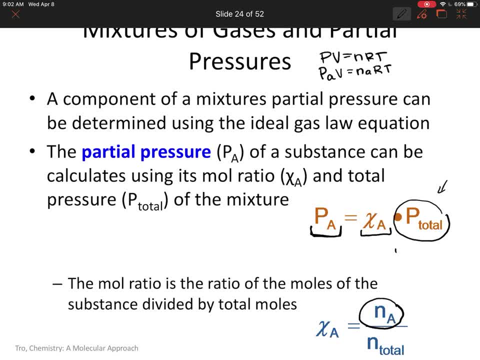 of the substances or the mass or other information, applying different things you've learned thus far. you can find mole ratio, Or you can even apply ideal gas to find the partial pressure of a substance, and just look for different things in this equation that you need to solve for. 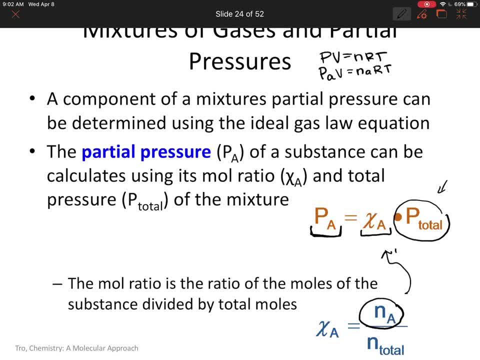 applying this, et cetera. I'm mentioning these things just because it's not. sometimes it's black and white. it's kind of puzzling the different things together for a bigger picture And with that said, let's practice. But before we do that actually, 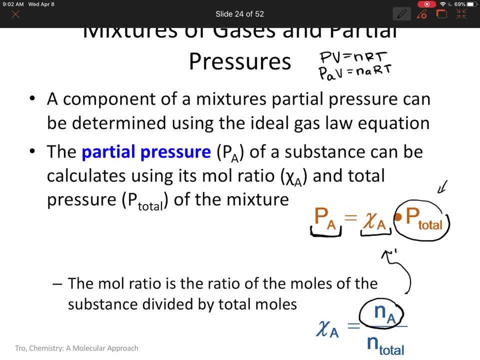 I want to go over one more thing. So what I want to say is where this comes from. because you know that a mole fraction is the number of moles of component A and the total moles of a sample, And because we can apply this, let's just say that: 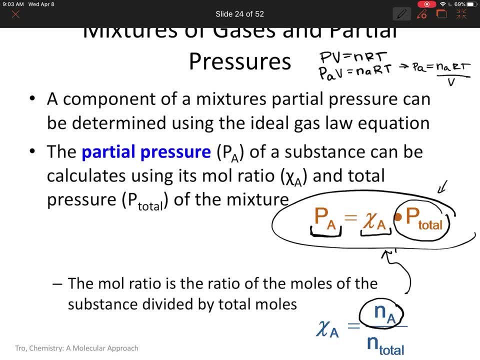 if I rearranged this to have, PA is equal to NA, RT over VA or V. right Well, RT and V, the volume, the temperature and the gas constant do not change of your total pressure and your pressure component. It is the number of particles. 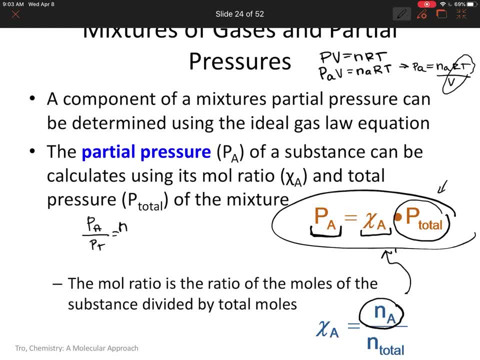 and the pressure that are changing. So if you wanted to know the ratio PA over PT, it would be the NA RT over V over N total RT over V, which then would give us just that the pressure of a substance over the total pressure is equal to. 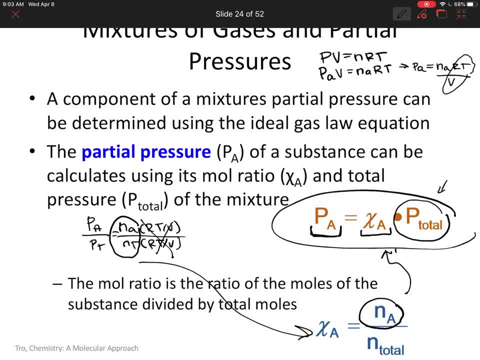 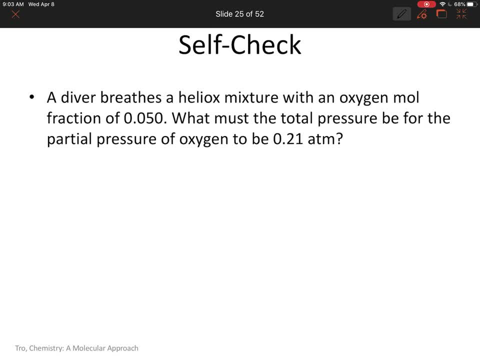 the moles of that particle over the total moles, which is therefore the mole fraction. Just showing you a little bit of the derivation where partial pressure and mole fraction are coming from. A driver breathes a heliox mixture with an oxygen. mole fraction of 0.050.. 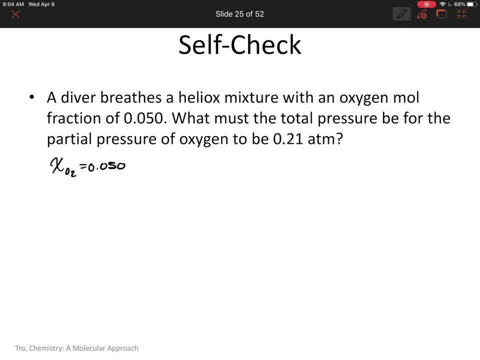 Okay, I'm gonna stop there. So I have oxygen mole fraction of 0.050.. What must be the total pressure? So I'm looking for PT- I don't know this- For the partial pressure of oxygen to be 0.21.. 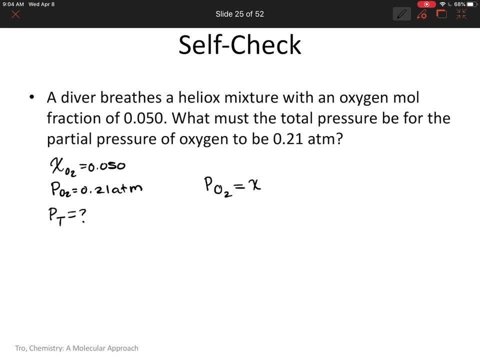 So I'm given my partial pressure, I'm given my mole fraction, I want my total pressure. Well, I know that partial pressure of a substance relates to the mole fraction of that substance times the total pressure. So if I'm looking for my total pressure, 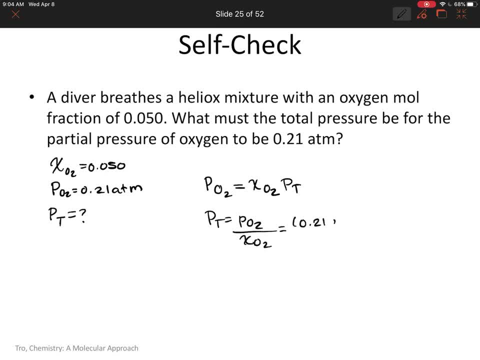 I would rearrange my equation to look for the ratio of the partial pressure and mole fraction and then plug everything in. Note how the mole fraction is unitless because it's moles divided by moles, which would cancel out And you would be left with just atmospheres. 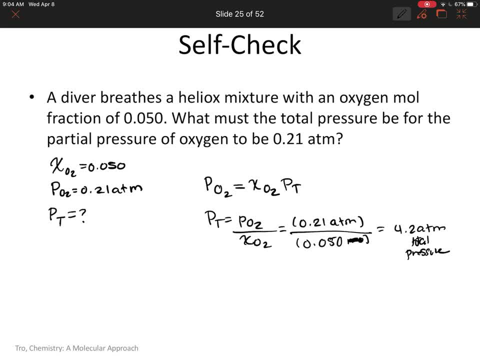 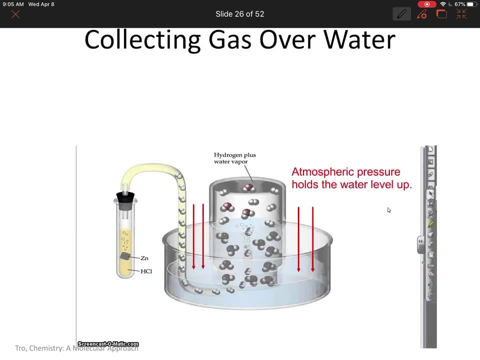 And you're in to be 4.2 atmospheres total pressure. Alrighty, last little bit, for the partial pressure is also talking about vapor pressure And vapor is steam, right, So this happens when there's bubbling going on. So look at this little diagram here. 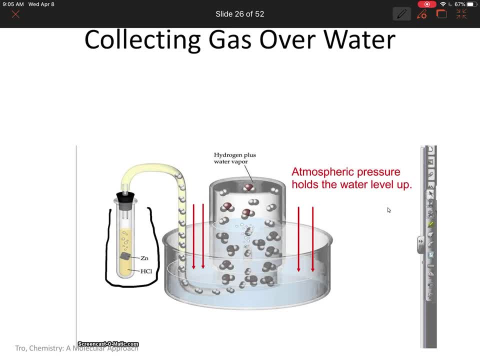 Know how you have this test tube, where you have this desired sample. Right, You have zinc. So what you did is you placed zinc into a test tube that has hydrochloric acid in it, And what that does is the zinc will react with the chlorine. 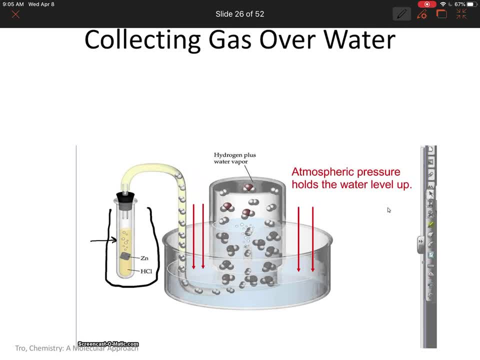 to form an aqueous substance and produce hydrogen gas. So these bubbles that you see are hydrogen gas. And so, through this apparatus, what happens is through our manometer, the U-shaped tube, the hydrogen gas particles are collected, And then through an inverted beaker. 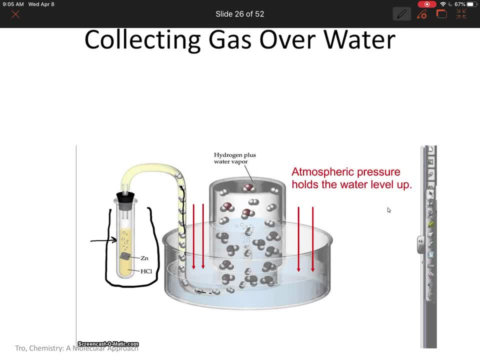 you can actually find the number of gas particles that can be obtained. So when the desired product of a chemical is a gas, the gas can often be collected by the displacement of water. As the hydrogen gas forms in this reaction, it bubbles through the water and it 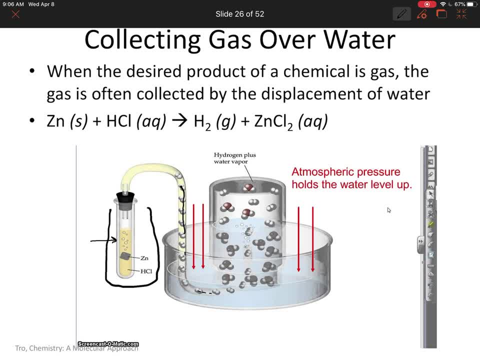 gathers in the collection of the flask. So you can see that we have all of these, The water molecules that are being gathered, and that the atmospheric pressure holds the water level to a certain spot because it's pushing down. So, based off of this difference between where the water level 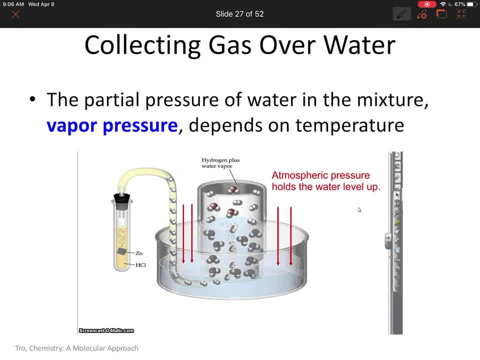 started and where it's ending, we can calculate the displacement of the molecules. The hydrogen gas collected in this way is not pure because there is water, So you have to account for the water molecules in it. It is mixed with the water, The water vapor, because some of the water molecules evaporate. 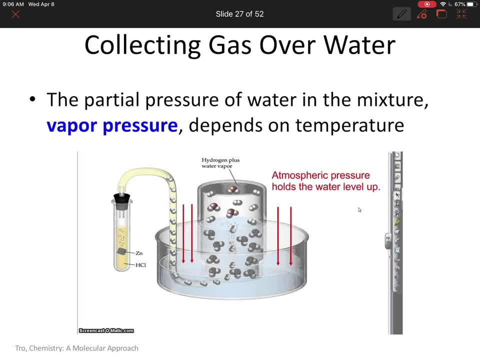 and combine with the hydrogen molecules. So you can't. it's not just water, It's not pure hydrogen. Some of them do mix. sometimes. The partial pressure of water in the mixture depends on the temperature, which is called its vapor pressure. 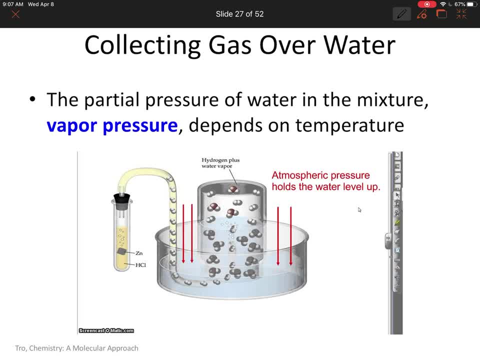 And just to know that, since this has to do with bubbling and a reaction and vapor, because of the steam of the water it increases. It's not just the vapor pressure, It's the vapor pressure of the water molecules. So this is what we can do with increasing temperatures. 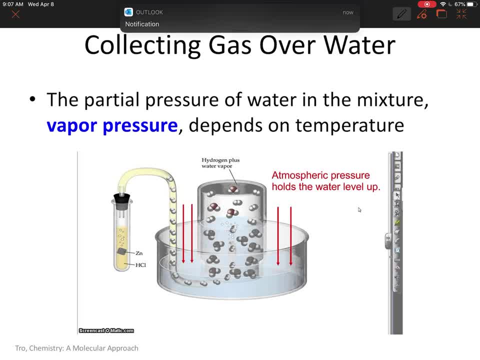 because higher temperatures causes more water molecules to evaporate. So then we can collect the hydrogen over water by saying: all right, well, my pressure total is equal to my pressure, hydrogen plus my partial pressure of water. Well, my partial pressure of water is known. 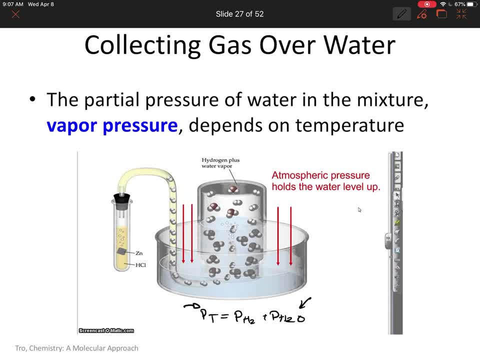 There's a table with different partial pressures of water particles collected in its vapor at certain temperatures and the total pressure you can calculate. So therefore, if you know these two, you can then calculate the partial pressure of hydrogen by subtracting the total pressure minus the vapor. 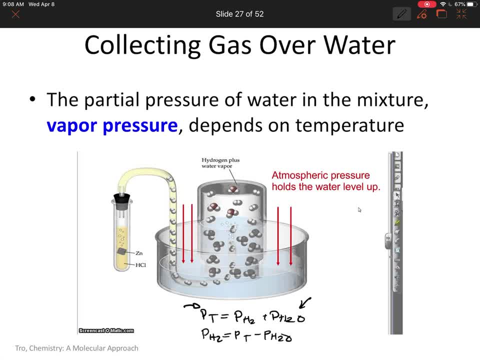 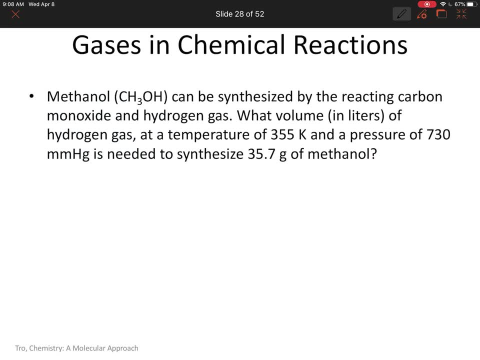 pressure of water. So in this way we can determine the exact pressure of a hydrogen mixture from a desired reaction. that's happening Now putting this all into a reaction, so all of the different rules and concepts we've learned so far can apply to gases as well. 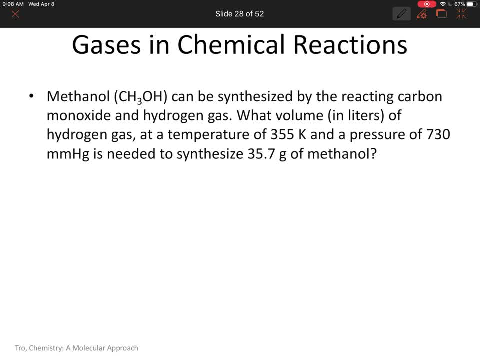 And the best way, rather than just writing out a bunch of definitions and steps, is to learn through a problem. So methanol can be synthesized by reacting carbon monoxide and hydrogen gas. What volume in liters of hydrogen gas at a temperature of 355 Kelvin and a pressure? 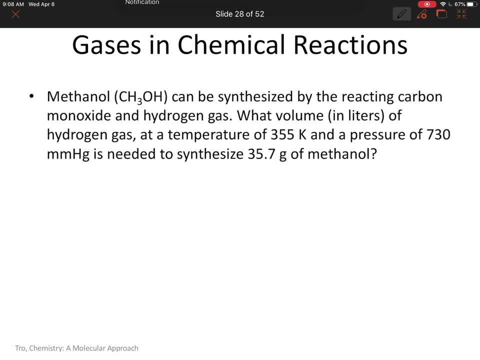 of 730 millimeter mercury is needed to synthesize 35.7 grams of methanol. So let's just write here what I'm given. So I have. I'm going to write it up here. given what volume of hydrogen gas at a temperature. 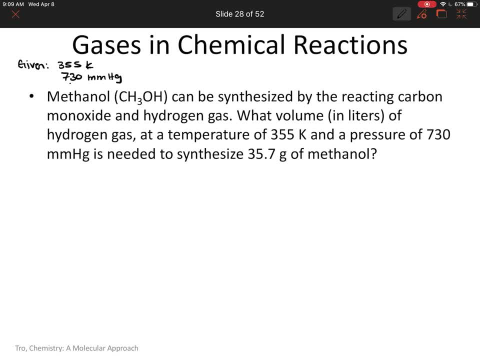 so I have a temperature of 355 Kelvin, a pressure of 730 millimeter mercury and 35.7 grams. So I want volume. but now exactly of what? So what? volume of hydrogen gas. So I want volume of H2 at a temperature of 355 Kelvin. 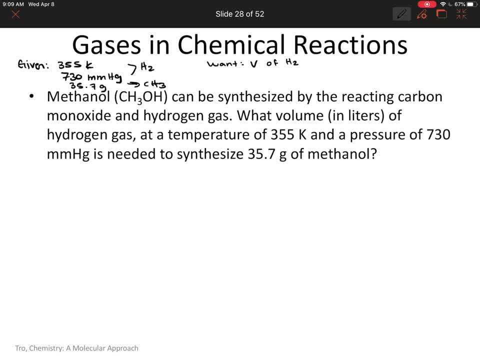 and a pressure of 730.. So these are also of hydrogen gas, but the mass is for methanol. So immediately I notice that I have information of one substance And I'm trying, And of another And I want to know the volume of hydrogen gas. 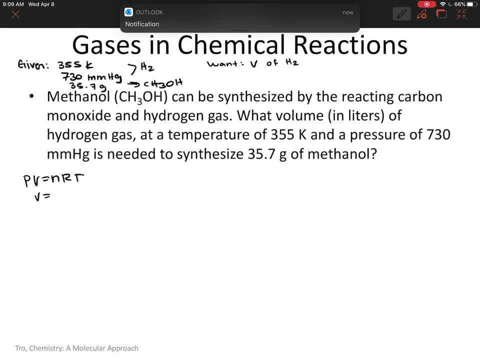 Well, if I'm given temperature and pressure and I want volume, I would think: well, I know ideal gas law And I know that I can find my volume based off of the moles, the gas constant, the temperature and the pressure. 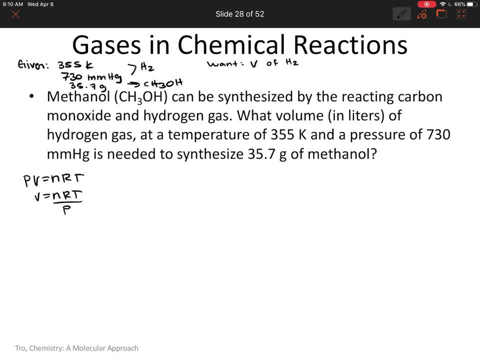 But what am I missing here? What do I not have? yet I don't have my moles. This is unknown, So I first have to solve for my moles of hydrogen gas. Well, I'm still given a piece of information. 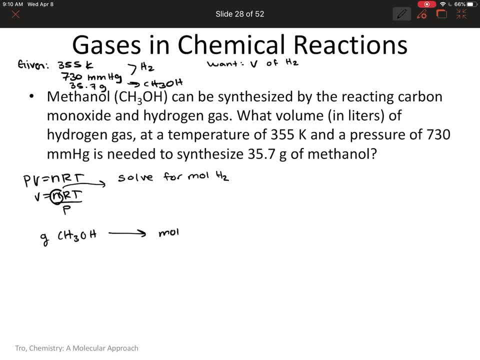 I'm given the mass of methanol, but I need moles of H2. Can I get there? Yup, because I know that I can go to moles of methanol using molar mass. And last, I need a study for this. So what happens at H2, will I get this? I get this Over and over. You can try to add an industry-like literature. Places like this are not습니다 to companies- stearium, but it's not easy to chickens, to warehouse workers standing. 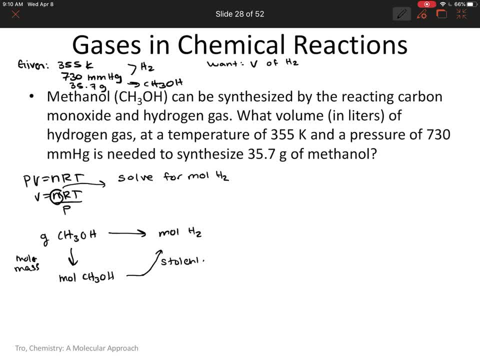 or labor groups, organization or labor groups. what are the problems? How can we другие includesent mehrere point units or high quintenter depletes? Why is itiad cutting? calculate passive activity And from there I can go to moles of H2 using stoichiometry. 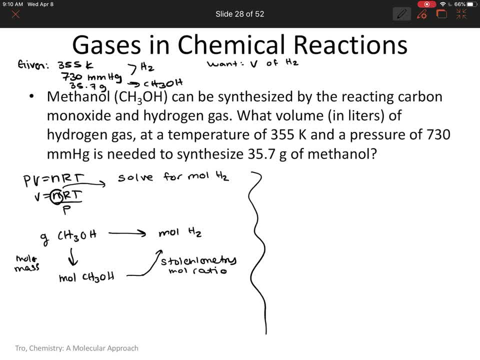 So if I need to use stoichiometry mole ratio, what should I do? I have to write my equation So it tells you that methanol is synthesized from carbon monoxide and hydrogen gas. So the reaction of synthesis is A and B coming together to form AB. 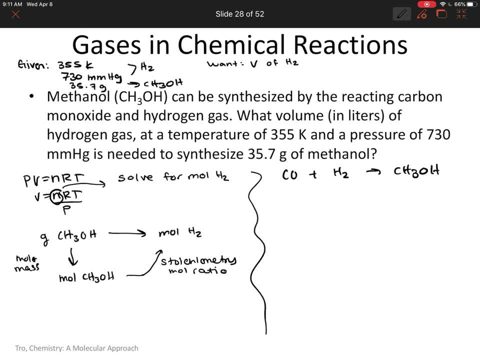 So that means we have carbon monoxide plus H2 to make methanol. Now take a moment to try and balance this equation. We need two here And now. I have enough to start, So 35.7 grams of methanol. Well, I already kind of wrote myself a plan here. 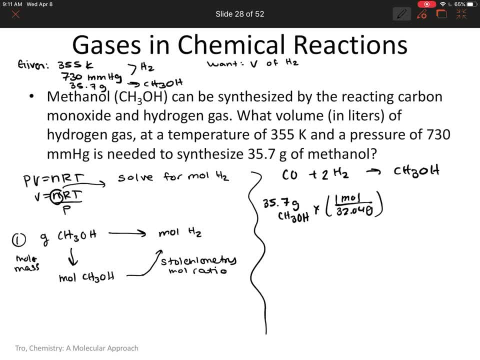 I have to convert to moles using molar mass, And then I have to use my ratio, So two moles H2 over one mole methanol, And that gives me 2.22 moles H2.. Awesome, And now I can go to my ideal gas, because I have all my other information. 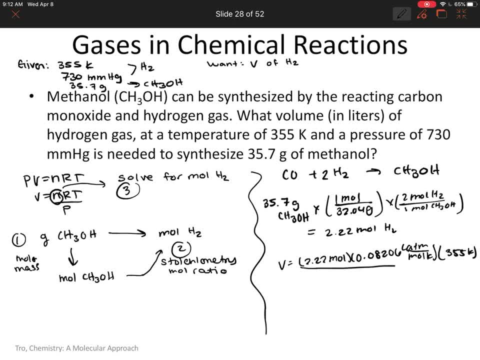 Making sure you convert the appropriate unit. So I already did it. We already know that we have Kelvin, And then we just need to convert the pressure to AB, And then we just need to convert the pressure to AB. So we have atmospheres, because our gas constant is in atmospheres. 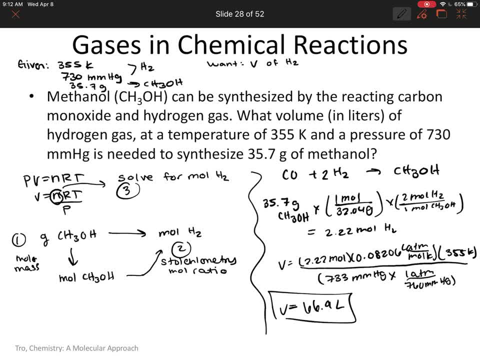 You plug everything in and you will get 66.9 liters. So using a couple different concepts to find your overall goal. knowing, kind of making yourself a plan like: what do you have, but what do those represent? Do they all represent one substance? 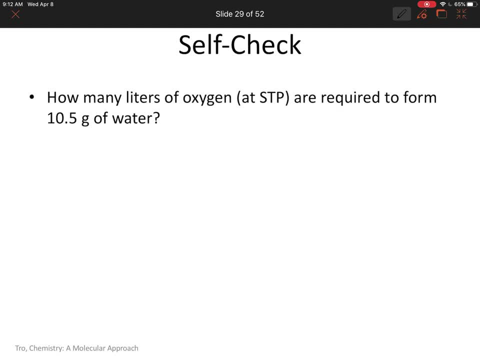 Do they represent multiple substances? What do you need? How can you get there? A couple little self-check problems: How many liters of oxygen are required to form 10.5 grams of water at STP. So what do I know at STP? 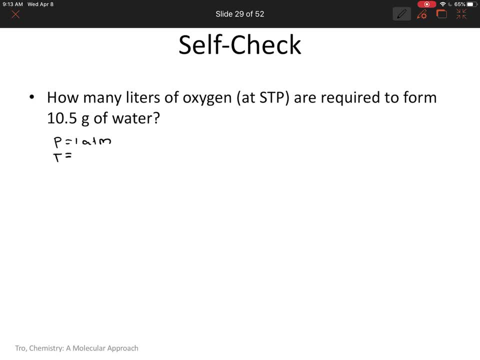 I know that I have a pressure of 1 atmospheres and I have a temperature of 273.15 Kelvin and I want liters. so I want volume And I'm also given my mass of 10.5 grams. Well, I know I can use my ideal gas. 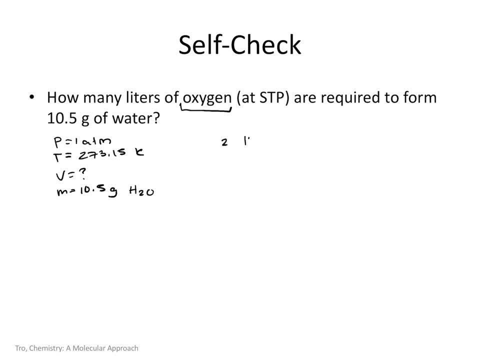 However, I want to know oxygen and I'm given the mass, So I'm going to need to write myself an equation And then I can do the same exact process that I just did, So since I'm given all this information of O2,. 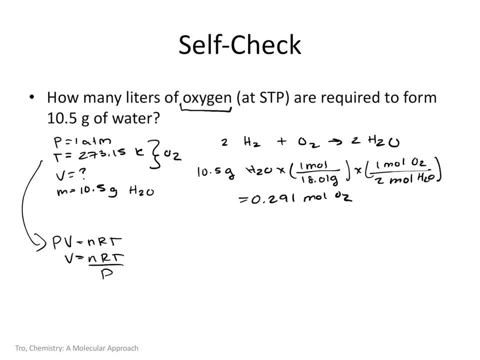 I know that I can use. PV is equal to nRT, V is equal to nRT over P to get my volume, But I need moles, O2.. I don't have that yet, Since I'm given my mass of water. 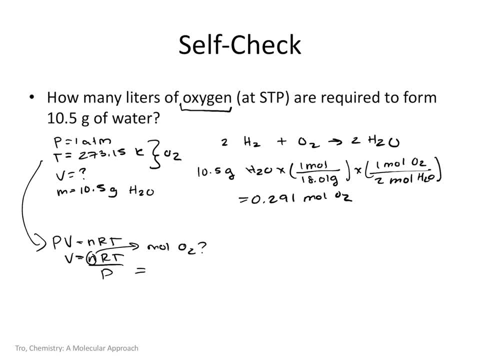 I can use all the different applications. I already know molar mass and mole ratio to get that amount. So then I can just plug everything in And then I can do my mass of water and I can use my mass of water. 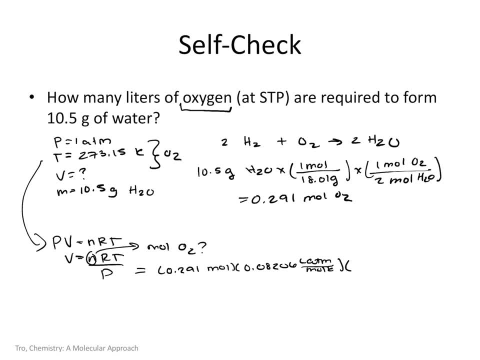 and I'm just going to keep doing the same thing that I did. All right, So I've already got my mass value, And then I'm going to use this energy. All right, And then I'm going to do my mass of water. 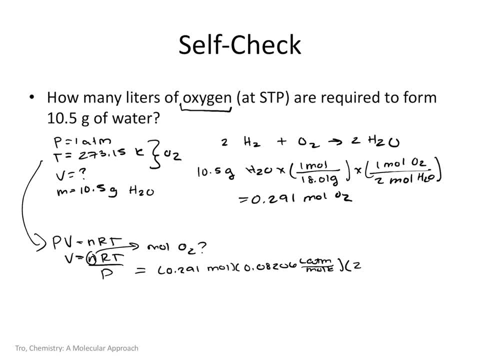 and I'm going to use the energy that I got from the stream to get my mass value. So basically I will put my mass value in this mass. So then you can see at the bottom of the screen I've got a small number here. 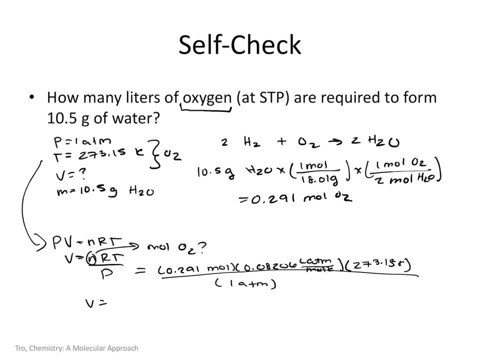 And I'm going to put that in here as well, to figure out the mass value. and that's all I've got. So I'm going to put that in here as well. and then, if you plug everything in, you would get 6.5, 2 liters and you're done. 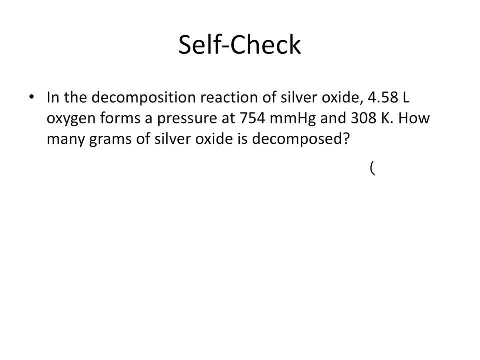 in the decomposition reaction of silver oxide. 4.58 liters oxygen forms a pressure of 754 millimeter mercury and 308 Kelvin. how many grams of silver oxide is decomposed? so we have a volume of 4.8 liters. 4.58 liters of silver oxide, so Ag2O and- oh wait, in the decomposition of. 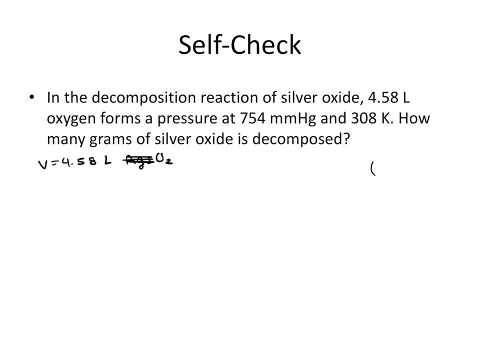 silver oxide 4.58 liters of oxygen forms. so we just have O2, a pressure of 754 and 308 Kelvin. so we have P is 754 and then temperature is 308 Kelvin. how many grams of silver oxide do we have? okay, so I want to know grams of. 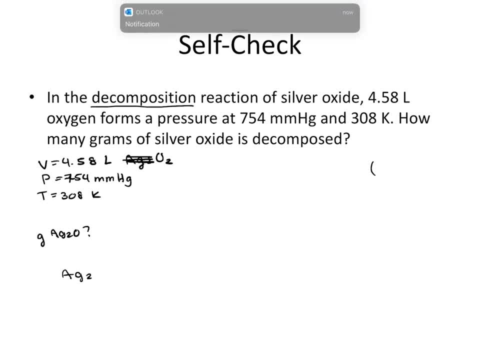 silver oxide. so let me write my equation. first, decomposition reaction. so that means Ag2O is decomposing to silver and oxygen and to balance we would need a 2 here and then a 4 here. awesome. so if I want the mass of this I can convert, since 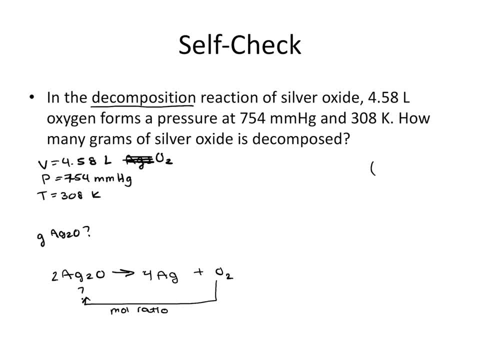 I have all this information from oxygen using my mole ratio. now I'm gonna let you try this one on your own, knowing that you have pressure volume and temperature, and since you know that ideal gas, if you have pressure volume, temperature, you can solve for the moles and kind of work. 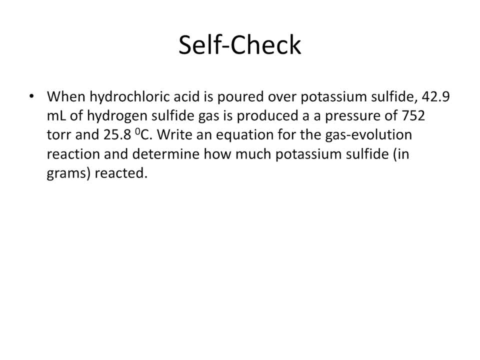 backwards to get the mass of silver oxide. when hydrochloric acid is poured over potassium sulfide, 42.9 milliliters of hydrogen sulfide gas is produced at a pressure of 752 torr and 25.8 degrees Celsius. write an equation for the gas evolution and determine how much potassium 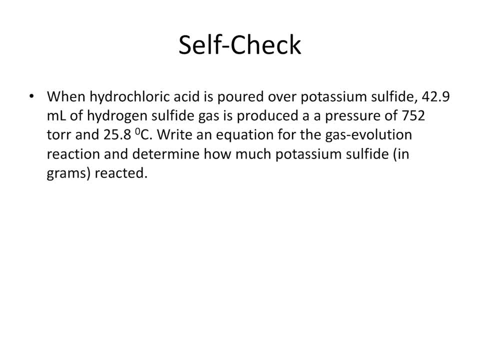 sulfide gets converted to oxygen. what's the reaction of the hydrogen to the graphite gas? well, wouldn't be a good thing to go for, and so we just take this equation and we take: is reacted. so this is going to be a little bit of your own practice problem.